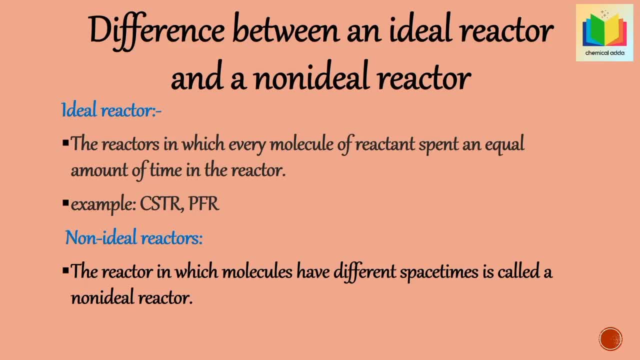 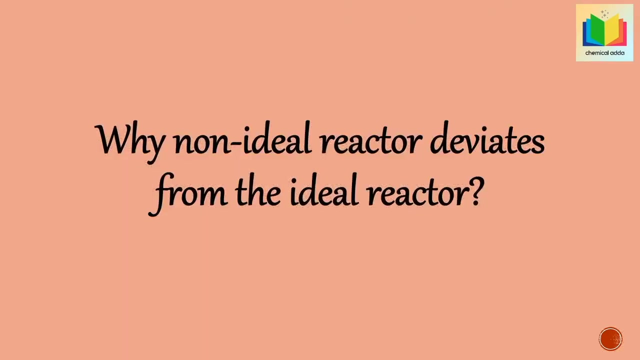 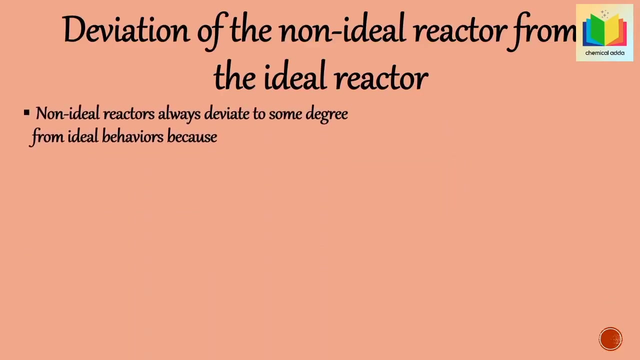 space-time. Hence non-ideal reactors are also called real reactor. This reactor never fully follows flow patterns and the behavior of a specific reactor mostly depends upon the extent of mixing. Now next question: Why non-ideal? non-ideal reactor deviates from the ideal reactor, So non-ideal reactors always deviate to some. 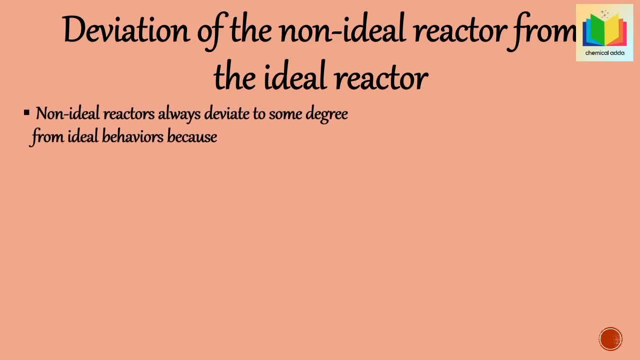 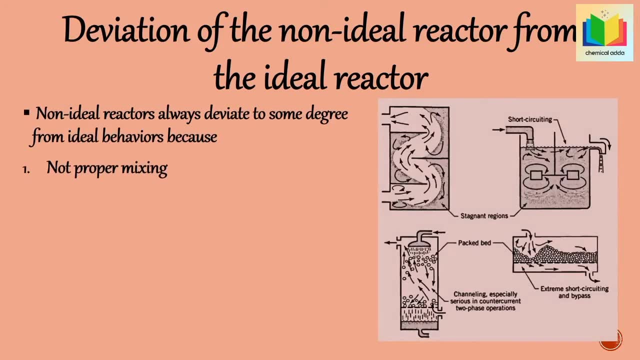 degree from ideal behaviors, because if there is no proper mixing, that's why the molecules of reactant do not spend an equal amount of time or space-time in the reactor. Next reason is by the creation of nearly stagnant regions in the vessel, So during the process, in some sections 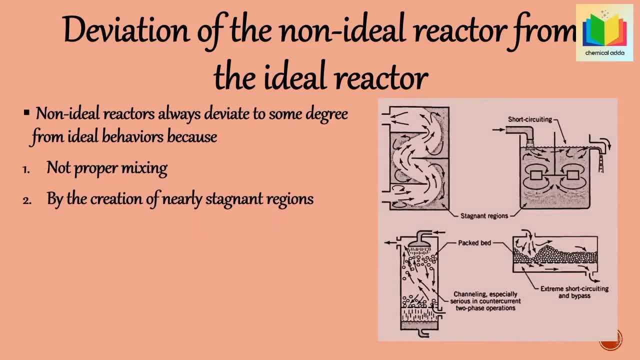 of the reactor, fluid flows very slowly or does not flow at all. Due to this, the effective volume available for reacting fluid reduces. This is shown in the first two figure. Next reason is by bypassing or short-circulating the fluid. 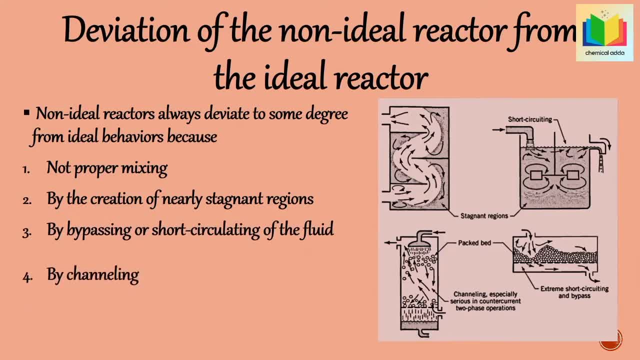 Next is by channeling. So in short-circuiting, the inlet fluid takes a shortcut route to the outlet without undergoing conversion in the bulk of the reactor. The same way channeling occurs in packed bed reactor, Then bypassing. So, in a packed bed, the inlet fluid bypasses the catalyst. 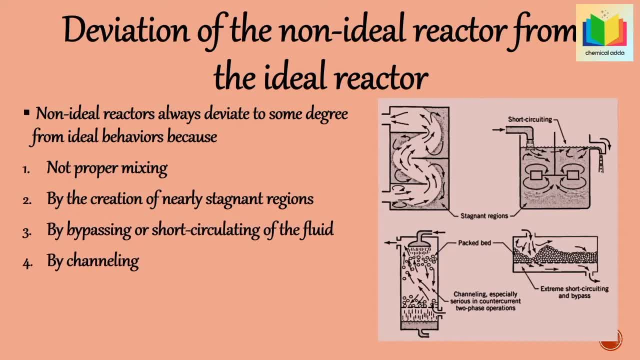 particles to the outlet. Next reason is by recycling. And last reason is due to vortices and turbulence at inlet and outlet. In plug floor reactor, at inlet or outlet, vortices and turbulence may be formed, which also affects the behavior of the. 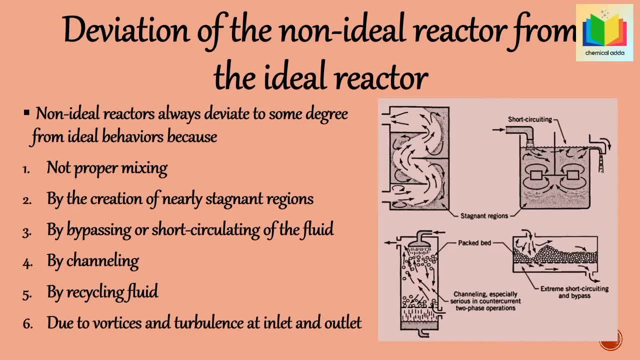 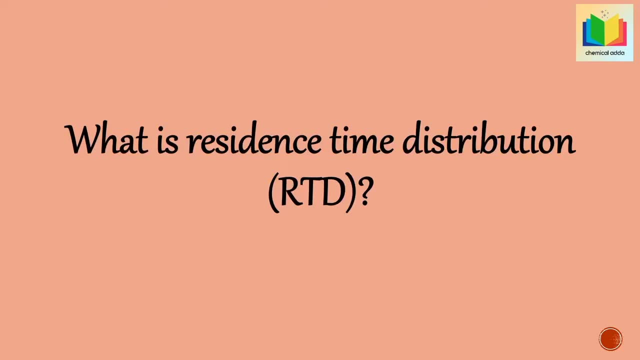 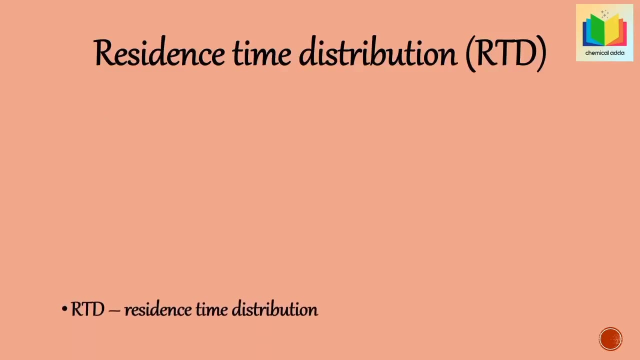 ideal reactor. Hence, because of all these reasons, the behavior of a non-ideal reactor deviates from the ideal reactor. Now next question: what is RTD, or residence time distribution? So full form of RTD is Residence Time Distribution. Hence, Residence Time Distribution is the time. 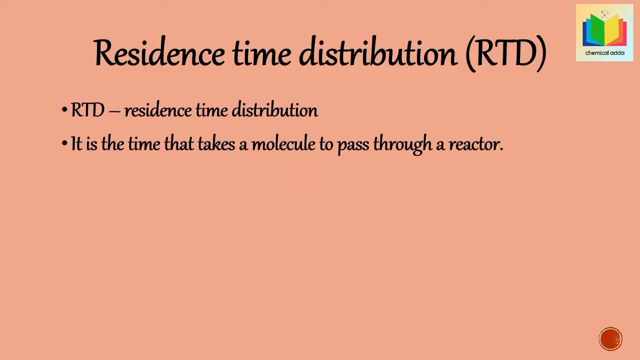 that takes a molecule to pass through a reactor. That means fluid molecule require time to pass from inlet to outlet or until a trip of some distance. This means that the time required to pass through the reactor is the time of distance, which is the time of time. 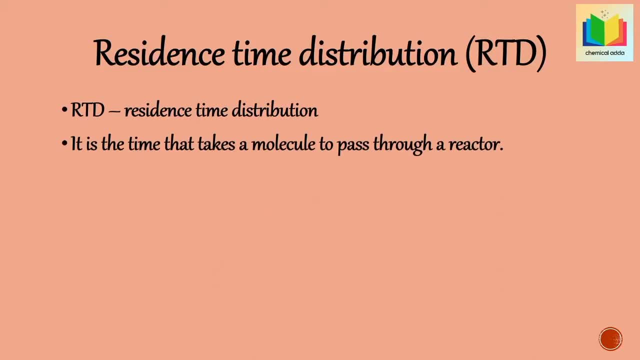 Hence this is the time of residence time distribution. Hence this time of residence time distribution. outlet of reactor. this time is called residence time distribution, hence from rtd we can tell that how long a particle stays in the reactor once entering in the reactor, then the distribution. 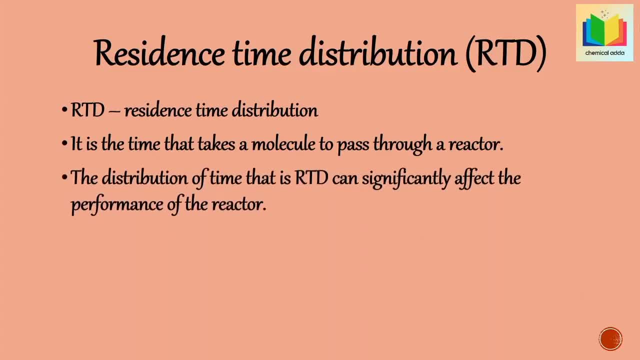 of time, that is, rtd, can significantly affect the performance of the reactor because, as we know, in an ideal plug flow reactor, all the molecules of material leaving the reactor have been inside it for exactly the same amount of time. similarly, in the ideal batch reactor, all the molecules of material within the reactor have been inside for the same length of time. 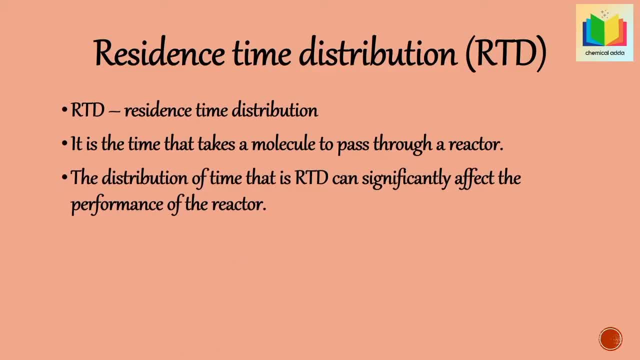 hence, in the ideal plug flow reactor and batch reactor, all the fluid elements have the same amount of time and the same amount of time, the same residence time. but for a mixed flow reactor, the feed introduced into it at any given time, then it is mixed with the material which is already present in the reactor. due to this, 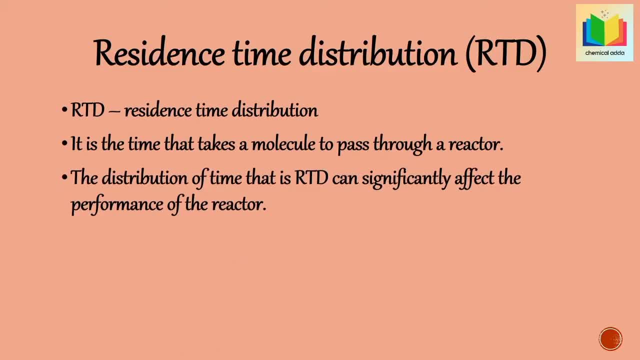 some molecules entering the mixed flow reactor leave immediately and other molecules remain in the reactor almost forever, because in cstr all the material has never withdrawn at one time for reactor. hence the distribution of time that is rtd can significantly affects the performance of the reactor. then the rtd of a reactor is: 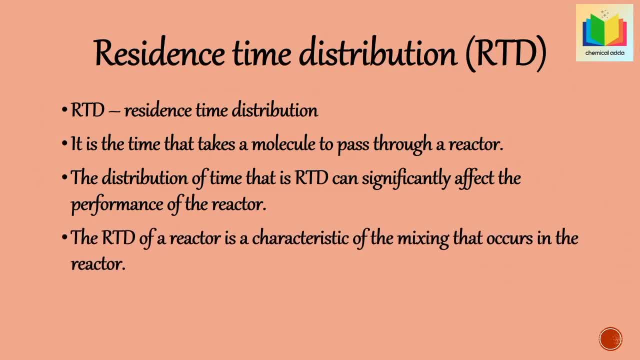 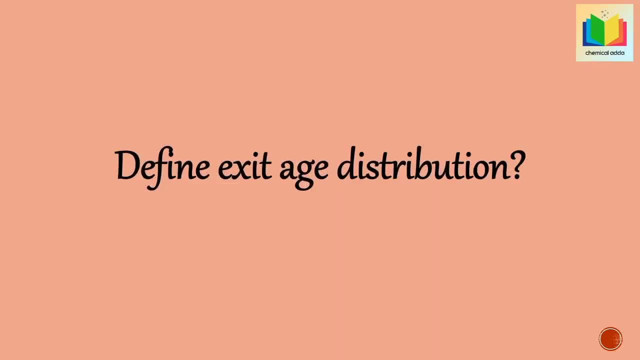 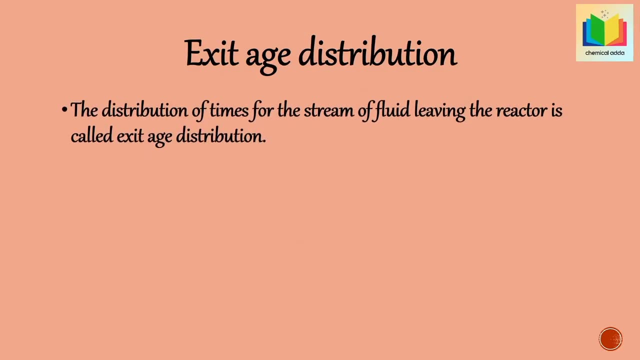 a characteristic of the mixing that occurs in the reactor. now next question: define exit age distribution. so the distribution of times for the stream of fluid leaving the reactor is called exit age distribution, as in the reactor every element of the fluid pass through different paths with different length of time. hence there is the distribution of these times for the stream. 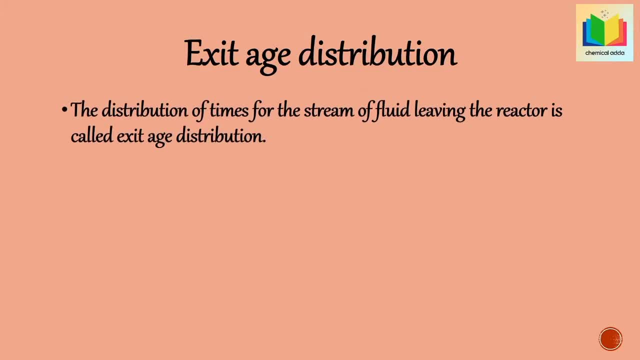 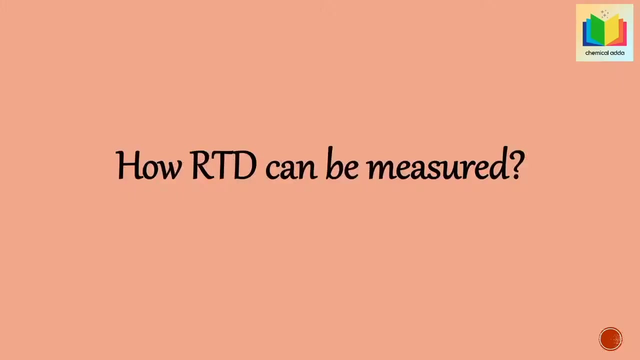 of fluid leaving the vessel. hence this time is called exit age distribution in the reactor. exit age distribution. it is also called residence time distribution. that is RTD. it is denoted by a. it has unit time inverse. now next question: how RTD can measured. RTD is determined experimentally by using an inert chemical as a tracer. so at some 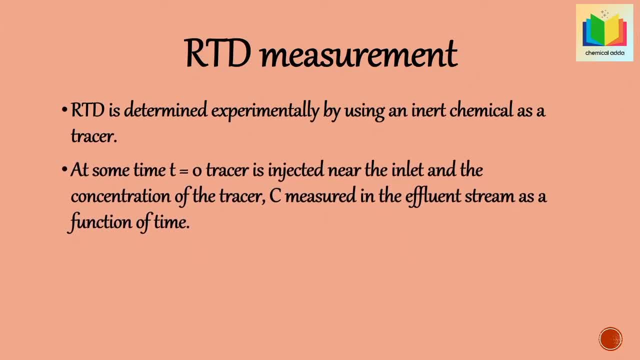 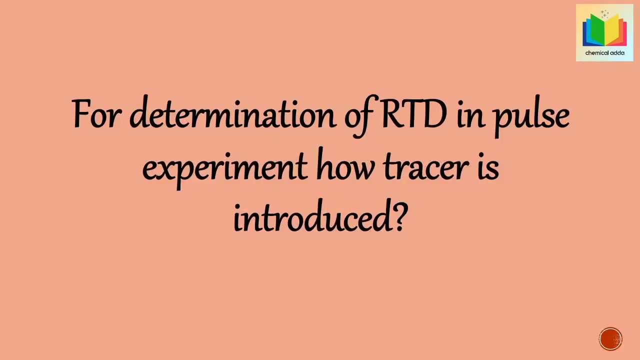 time T equals zero, tracer is injected near the inlet and the concentration of the tracer C measured in the effluent stream as a function of time. there are two methods for injecting the tracer. first one is pulse input. second is step input. now next question: for determination of RTD in pulse experiment, how tracer is. 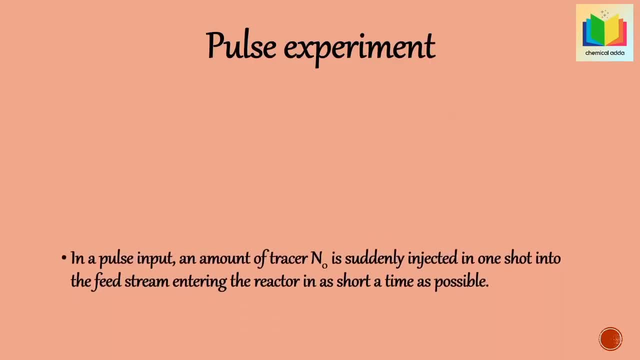 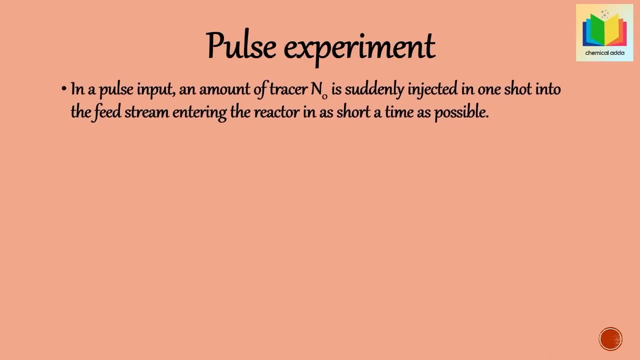 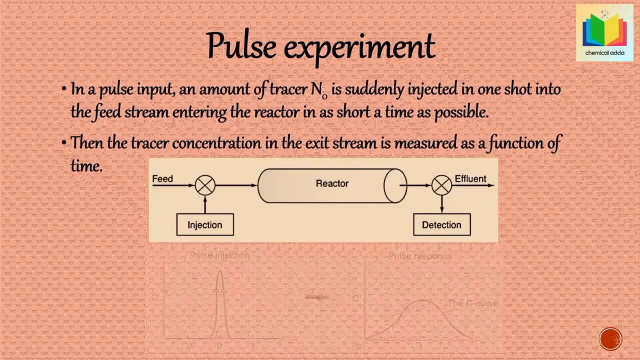 introduced. so in a pulse input, an amount of tracer and zero is suddenly injected in one shot into the feed stream, entering the reactor in as short time as possible. then the tracer concentration in the exit stream is measured as a function of time. the graph shows pulse injection. 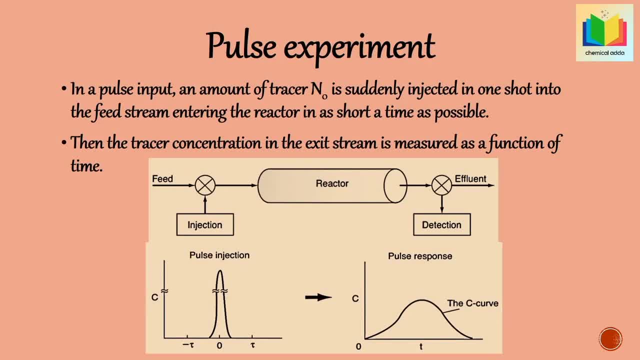 that is how concentration is changing with respect to time at the inlet of the vessel and the pulse response graph shows how concentration is changing with respect to time at the outlet of the vessel. the pulse response curve is called as C curve. from the pulse response we can see that 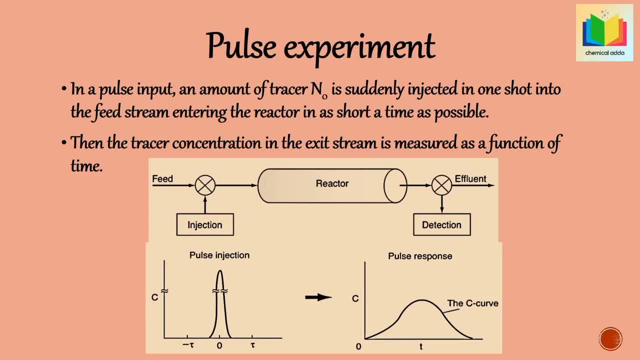 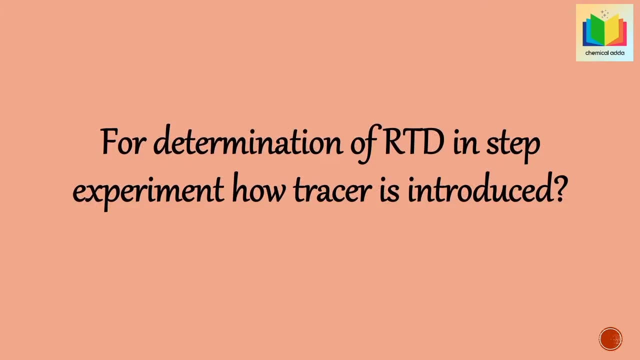 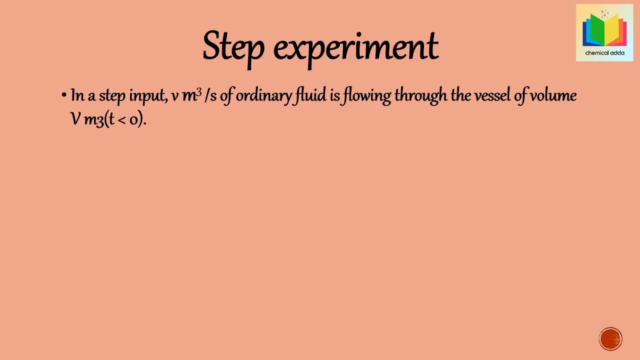 the concentration of tracer in the effluent stream increase with time, reaches a maximum value and then falls, which is approaching zero. now next question for determination of RTD in step experiment, how tracer is introduced so in a step input: V meter cube per second of ordinary fluid. 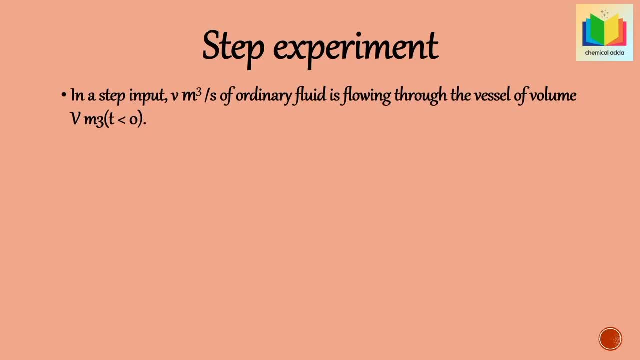 is flowing through the vessel of volume V meter cube in less than zero time. that is, T is less than zero, then at T is equal to zero. switch from ordinary fluid to fluid containing tracer with tracer concentration Cmax. that means at time zero. we start adding a small flow of a tracer. 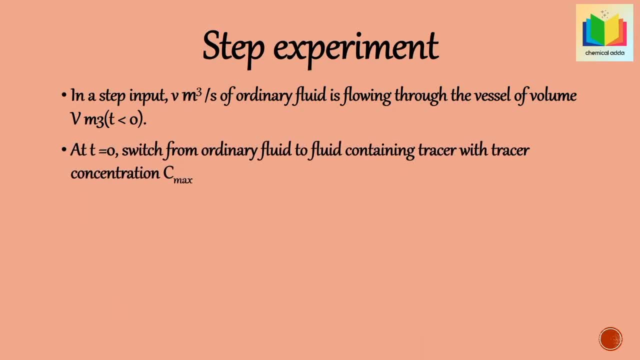 to the feed stream and measure the tracer concentration in the effluent stream. until after a long time it matches the concentration of the feed stream. then at the outlet, concentration of the tracer C step is measured as a function of time. until after a long time it matches the concentration of the feed stream. 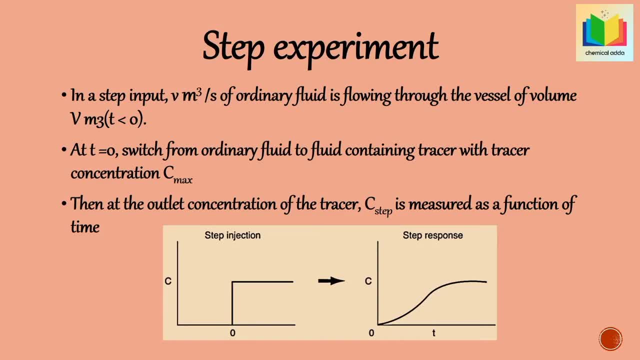 the advantage of this method is the total amount of tracer in the feed over the period of the test does not have to be known. but disadvantage is the concentration of tracer in the feed is sometimes difficult to maintain constant. even a large amount of tracer also required for this test. 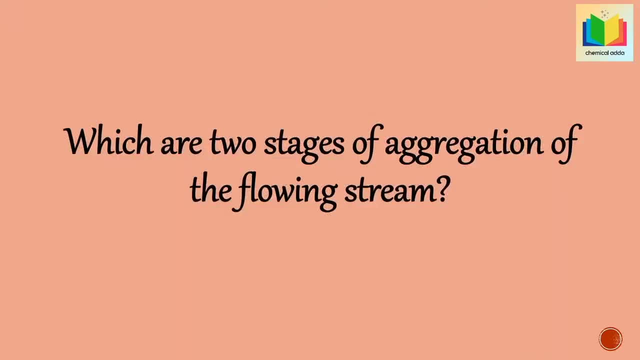 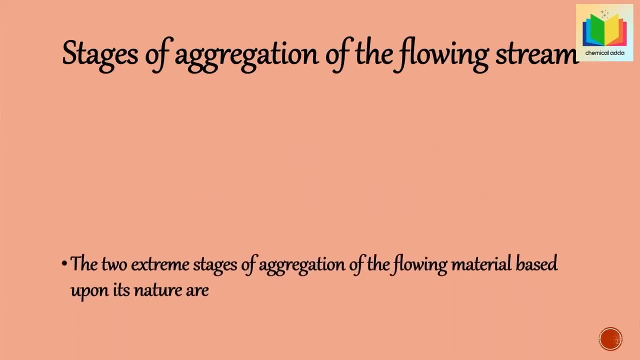 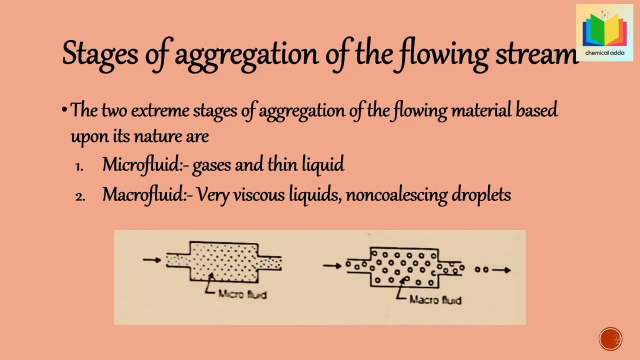 now next question, which are two stages of aggregation of the flowing stream. the two extreme stages of aggregation of the flowing material, based upon its nature, are microfluid and macrofluid. so microfluid, as the fluid in which molecules are free to move everywhere, collide in intermix. 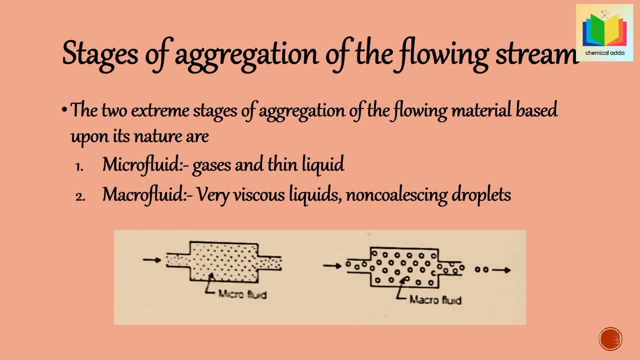 examples of microfluid are gases and thin liquid, as the molecules of microfluid are mix, collide and move everywhere. hence microfluid exhibits no segregation. now let's see macrofluid. so microfluid as the fluid in which globules or aggregates each contains a large number of molecules of a given age.